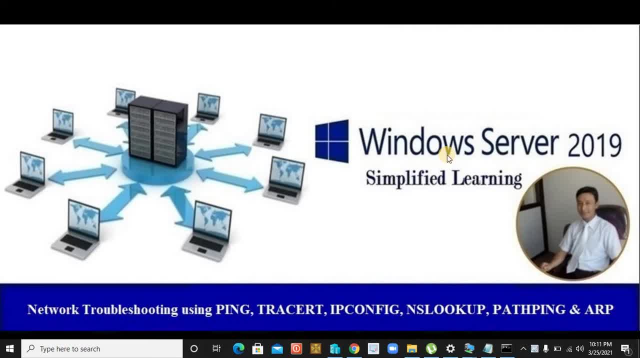 Hello, server 2019 system administration. Welcome back everybody. I'm Prakash Madan, your trainer for this entire series. So, as a system administrator or system engineer or any IT head, wherever we all work, one of the most important tasks in order to, you know, perform our day-to-day activity is 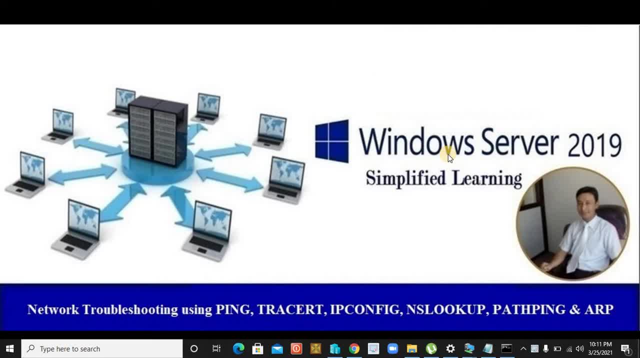 to troubleshoot your networking as well. So, apart from knowing all the group policies, okay, all the new features or the rules or the services that we are going to deploy in our any network environment and using any server family operating system, it is a major responsibility of that system. 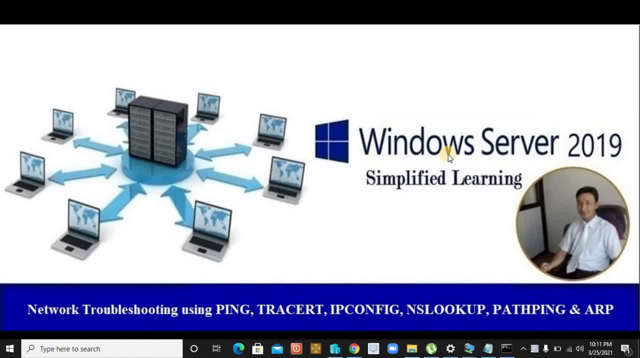 administrator to troubleshoot the network, And this network troubleshoot is the day-to-day activity of every system administrator. So, in order to help you to perform all these day-to-day activities, today I'm bringing this video to help you to clearly understand which are the most. 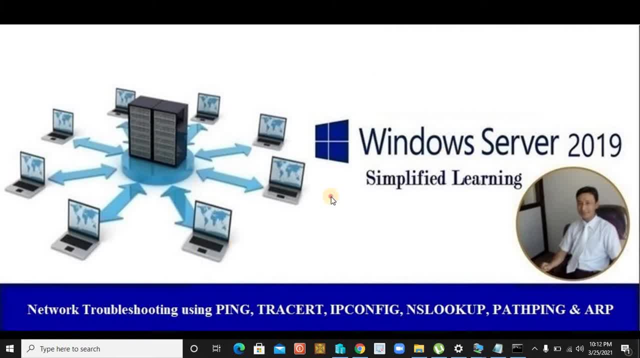 commonly used your command line tool utilities. So now, today, we are going to use some of the most important command line that will definitely help you to troubleshoot your network. So let's get started. So for that, I'd like to take you to the command from first. So let's go, And first we're going to. 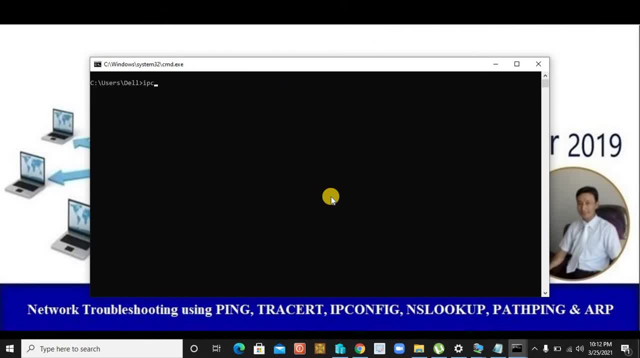 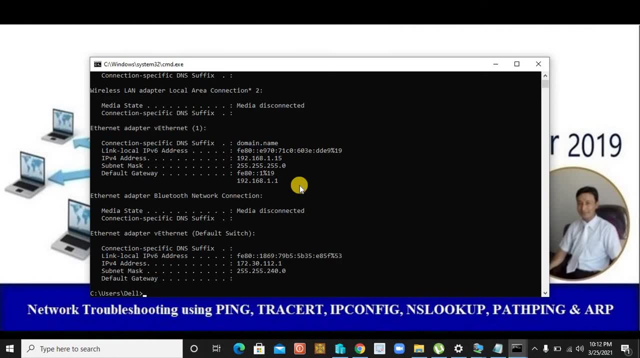 discuss about the use of this IP config. Okay, so let's say, if I use the hit the IP config, this command basically IP config. okay, this command shows you the IP configuration of your network properties. Actually, it may be your wireless, it may be your NIC, anything. okay, that means a. 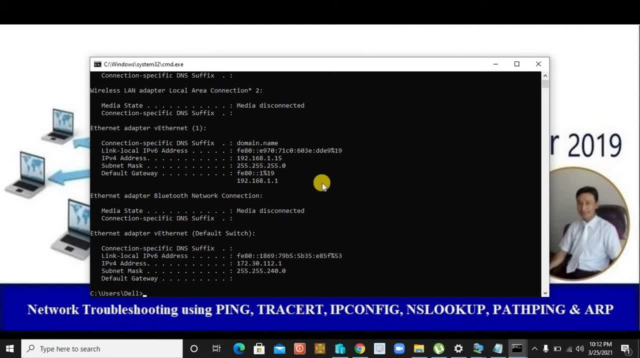 physical NIC. Now over here I hit IP config. if you notice over here it's showing me the IP address. Okay, this is my IP address And it's showing: 1.15 is my IP address And my subnet marks. is this? my default gateway is: 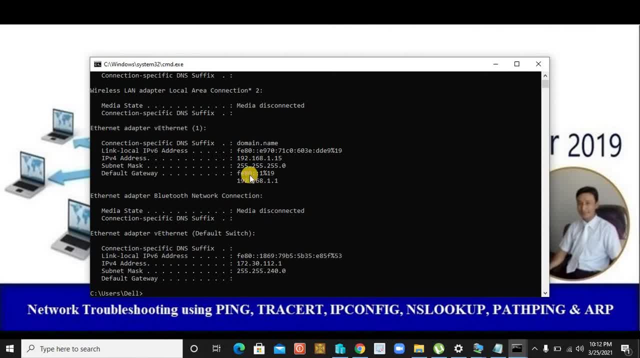 this. So these are the basic information that every system administrator go through in day-to-day life activities, But when we hit IP config, it will not show you the rest of the detailed information of this network properties. In order to see that, we're going to need to go to the 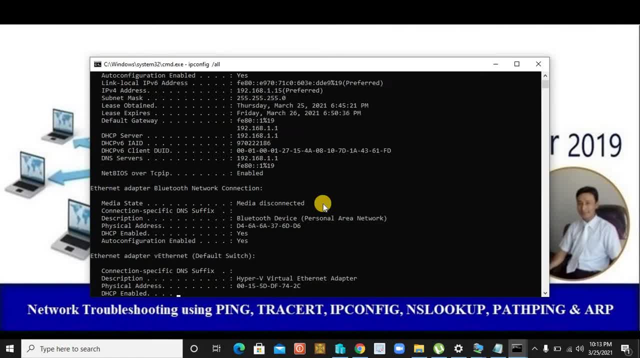 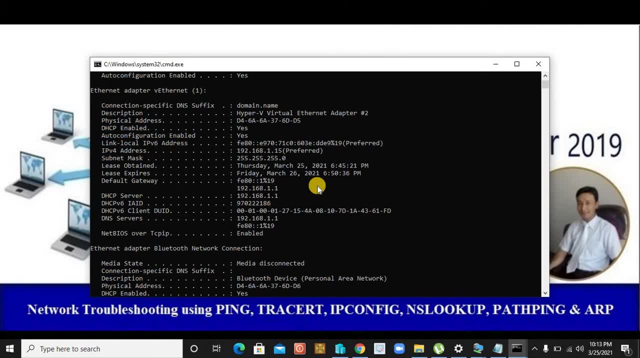 command that we need to hit this command: IP config slash alt. So when you hit IP config slash alt, you might have noticed, comparing to the previous command, it's showing me further more detail. That means your DNS information and your IP is a DHCP IP or not, and how long this IP is going to. 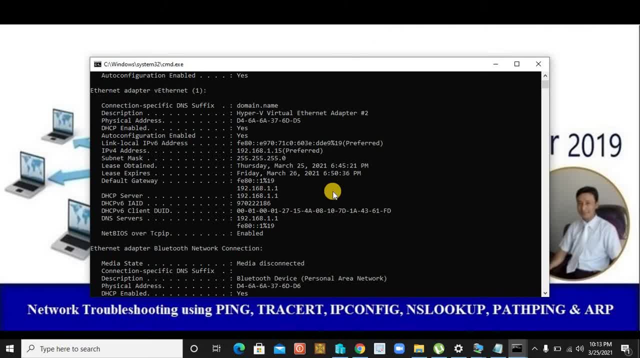 remain in your system. when this IP was obtained. when this IP is going to be expired, If you see over here, lease obtained is on this day, so and so your lease expired is on this so and so, whereas if I hit simply, 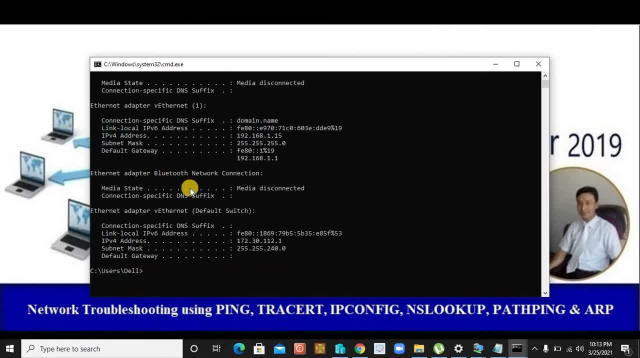 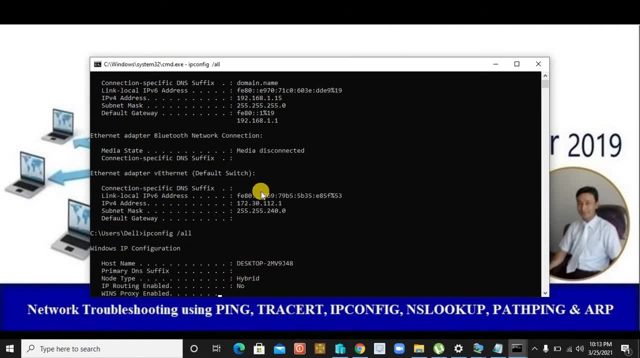 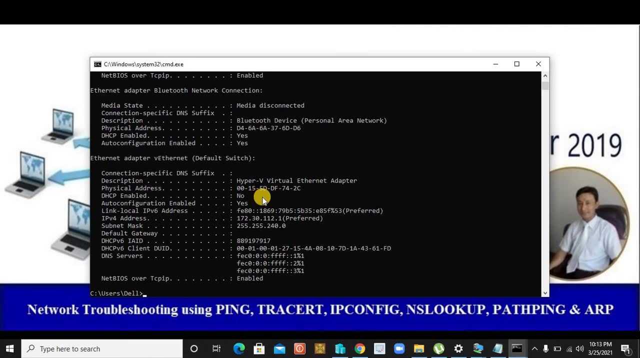 IP config, it is not going to display all of those information. See, there is no information about the DHCP. So if you'd like to see all the information okay about your network or NIC, in that case you'll have to go through the IP config slash alt, not only IP config, because IP config slash alt is. 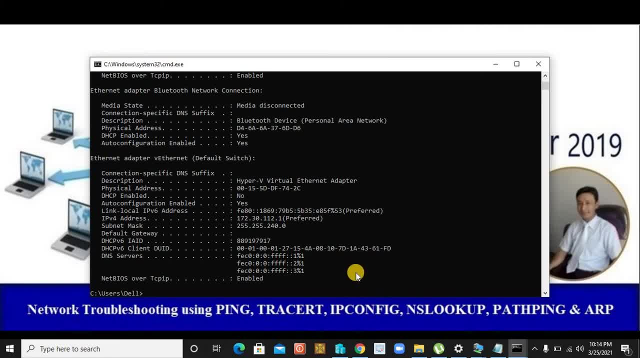 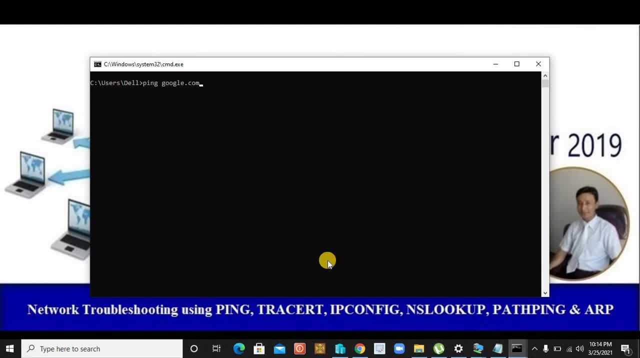 going to give you rest of the detailed information that cannot be seen simply hitting the IP config. Okay, now let's go to the next command, that is ping. This ping command is basically used to send your echo request. actually, That means it will send the echo request to your destination servo or destination- any device. 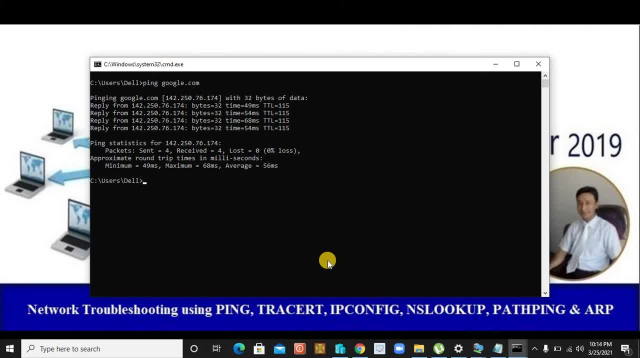 any IP and from where you're going to get written in response the echo requests only. So it's using the 32 bytes. If you notice, over here it took around 49 milliseconds. it sends four echo requests and it receives four only, If you notice. 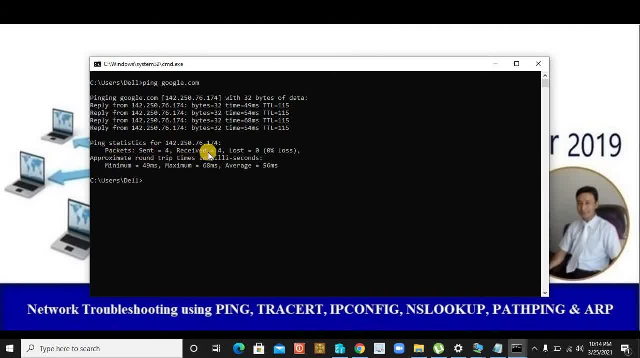 over here, the packet sent over here is a four and the receipt is also four and loss is zero. if you notice, over here it's taking 56 millisecond, since it has to go over the cloud, so it takes bit longer time in order to get the response from your google server, whereas if you are pinging. 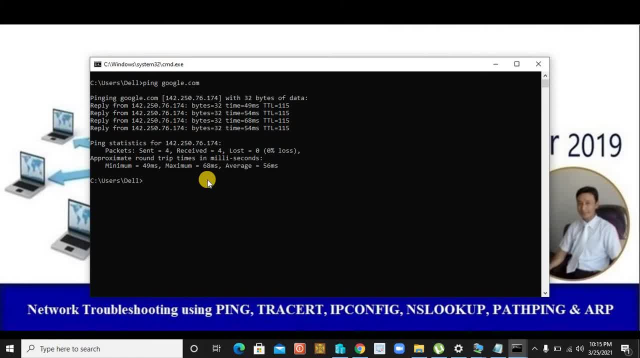 in your local area system if you are trying to ping any of your host or any of your server staying in your local area network. by that time you should be able to notice that this average time should be very less to the minimum, because we are not going to the long. 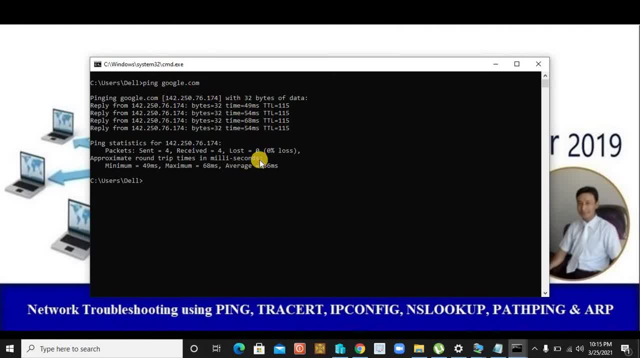 distance. so that's why this ping command is used: to actually test the connectivity to your device as well, through your website also. that means ping command is basically used just to test the connectivity between you and your destination server that might be your any website or that might be your any ip address. 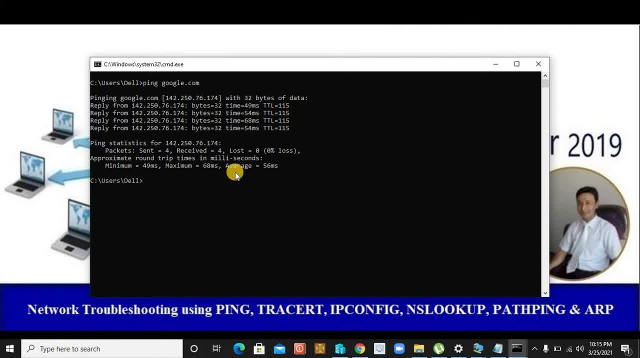 means when we hit the ping command and it replies in the 32 bytes and you have a zero loss. in that case you can surely assure that the connectivity between two devices are correctly done, whereas if, while pinging, if it does not return 32 bytes of your equal requests over here, then we should be. 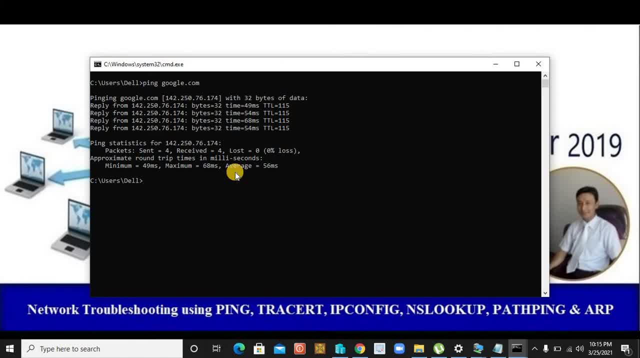 clearly able to understand that there is no connectivity, connectivity between two devices and that might be having certain your physical issues also, maybe your rg45 is having the issue, or somewhere your switch is turned off or somewhere your router might be turned off. so these are the common problem, that means the basic problem that we face as a system administrator in 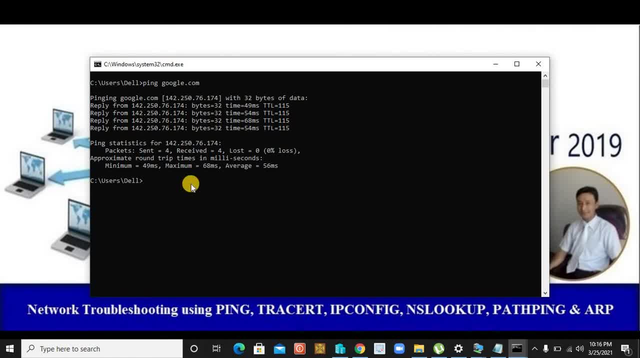 any network environment. so now let's go to the next command. okay, after ipconfig, ipconfig slash, solve and ping, we are going to talk about the nslookup now. nslookup, this command actually is fetch. it fetch the dns records for a given domain name. that means when i hit nslookup. 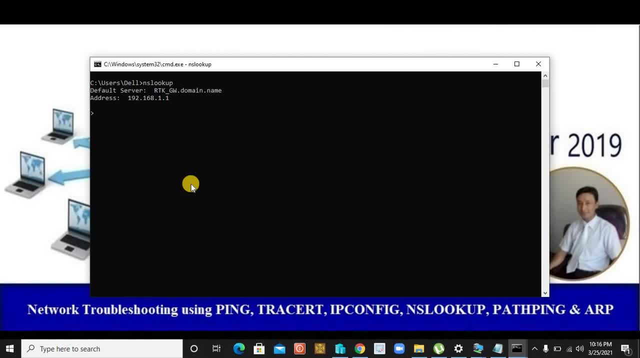 and i would like to go through the dns record of that domain. in that case it's going to show me the ip address insert, whereas if i do this- let's say first i'm going to ping it googlecom- it's responding from the one ip address, whereas if i would like to see the 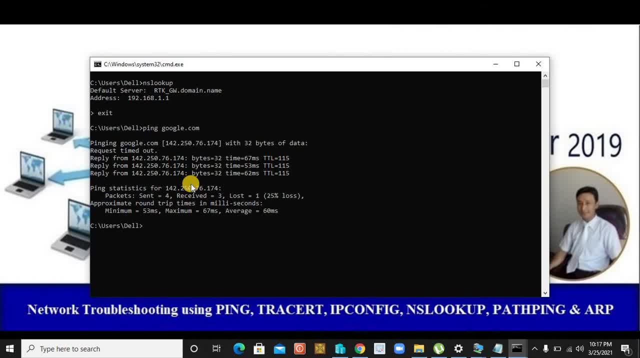 rest of the ip address through which i am going to communicate to this google. in that case, ping will not respond you using the multiple ips. if you would like to go through the multiple ip of google, in that case we can use nslookup command- nslookup. see, now these are the ip addresses you might. 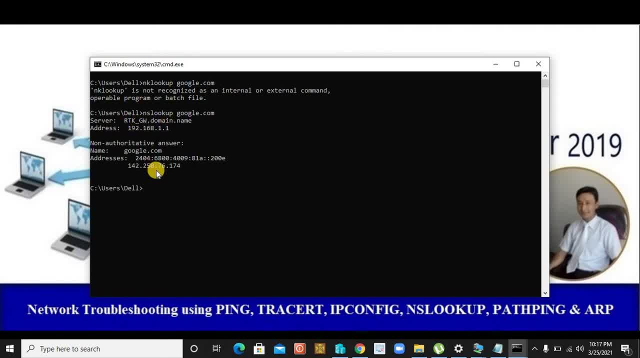 ip address is this: okay, it's a router one and this is the ip address. but if you are interested to see the rest of the ip address, dns records- okay, the dns records of google. you have a power of this nslookup command, so let's try that. 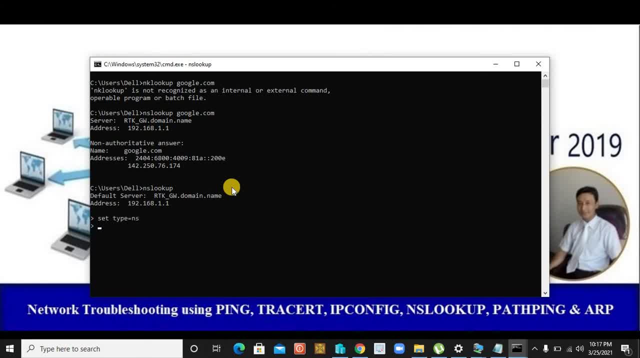 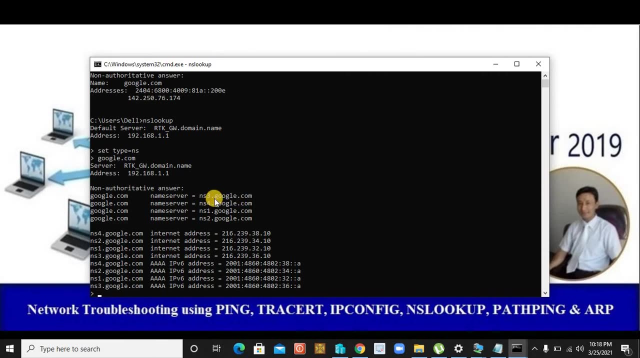 type is equals to. i write googlecom. now you'll find it will tell you the dns name as well as the ip address of this google. see. these all are the dns name actually: ns3.googlecom. it's a domain name actually, and they are using the different ip addresses, see. 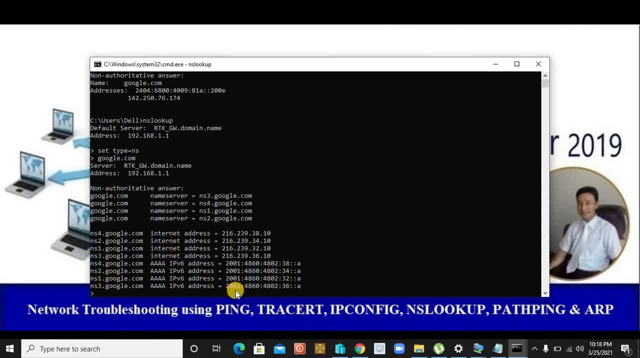 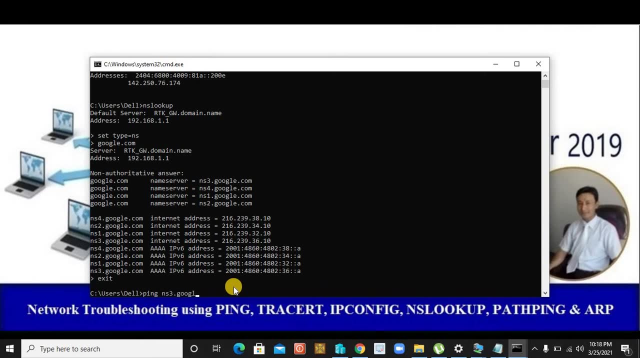 if you see over here, ns3, ns3, this is the ip address, whereas if i see you to show you the practical, i can ping this server using the name as well. it's a dns name. that means if i ping ns3, dns3.googlecom, that means this ip address should get respond. 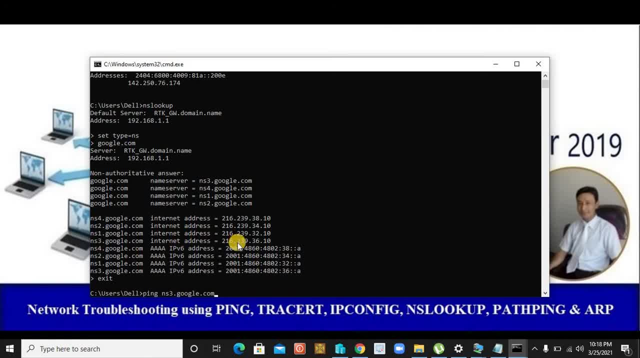 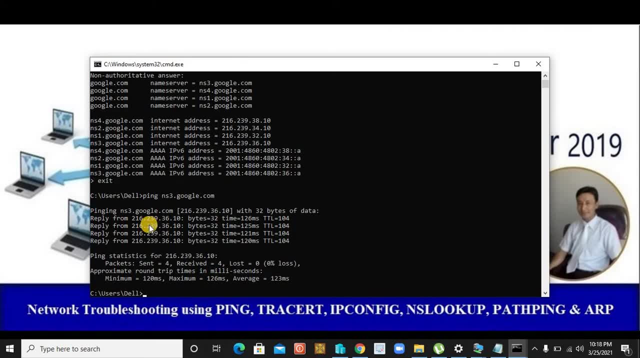 okay, that means this is ip version six and your ip version four is over here. it should reply particularly that ip address. only you see is exactly the same ip address, so it will help you to know the ip address address actually of your any DNS record. so apart from this, now the next command that we're going: 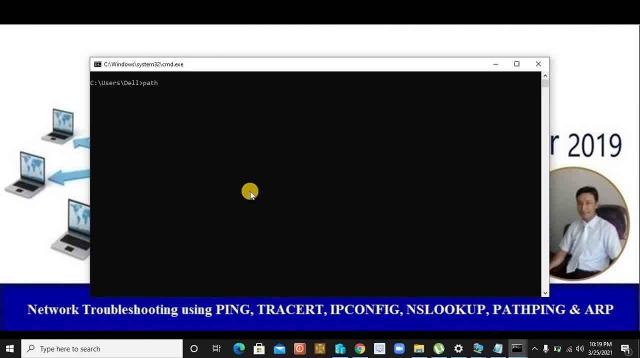 to discuss is about your path ping, let's say google. now, this path ping command is actually the combination of ping and the tracer. it helps you to find the location of a packet loss in a route between you and the host. so it's a combination of your- that means your ping and the tracer. okay, 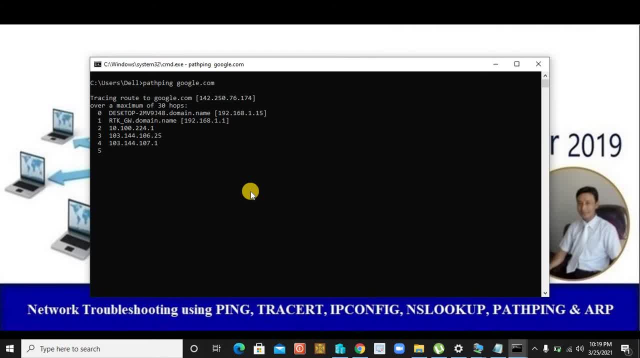 now. yeah, I might be having the slow internet disconnection so it might take time. so it will give you the detailed information actually before you reach to the googlecom. now. you see, by default the maximum hope count is the 30. this hope count means the number of total number of routers through. 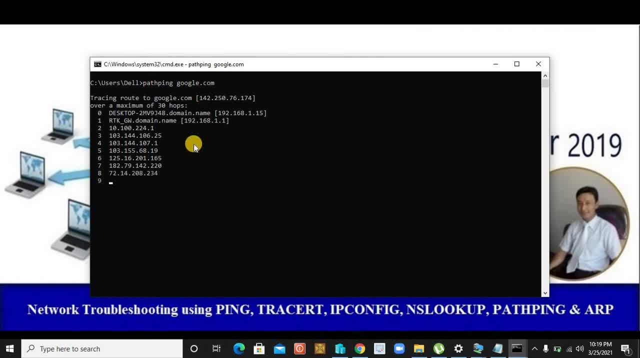 which you are going to pass. actually that means, if it says the 10 hopes, that means 10 routers. so first, when I hit pathping googlecom, the first request is coming out of my device itself. this is my device itself, and then it will go to my router and after that it will show you which are the 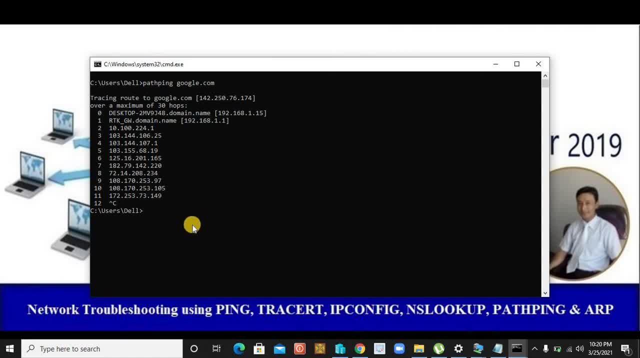 hopes. that means which are the routers through which you are passing through before you reach to your destination server. now, next important command is tracer. now tracer command is actually: it helps you to see step by step route of packet takes to the destination you specify. that means if I hit tracer googlecom now, it's going to show you all the hops. okay, all the hops that I have. 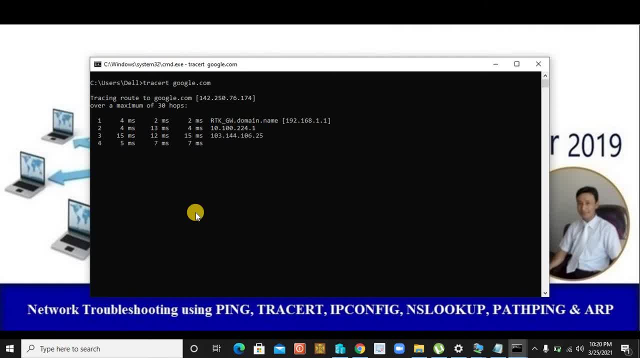 passed before I reach finally to my googlecom server, so it's showing how many milliseconds its taking. that means hop 1, 2, 3, 4, 5. it's passing more now before I reach finally the googlecom, how many pass? it's going to show me that information. 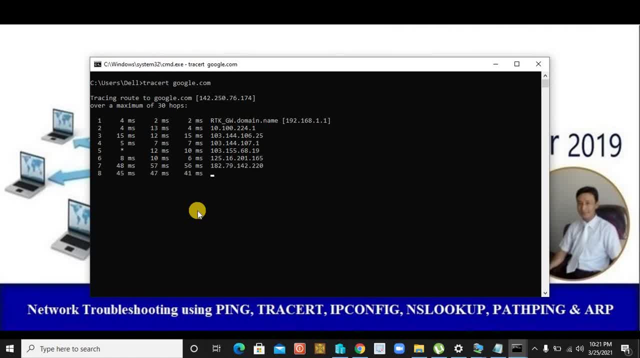 it's still counting, it's searching- so far we have passed over the eight hops before we reach to the googlecom- and it's returning you the ip addresses of those servers. that means those routers also. that means when i hit googlecom i passed from all of these routers which normally we 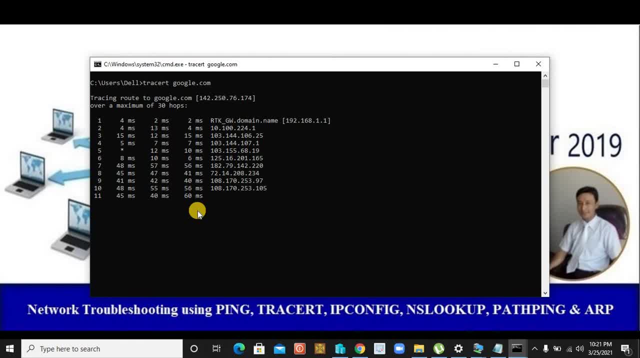 cannot see so this: in order to see this, all the information, you should have a proper knowledge of this command line tools, which i'm going to show you right now. so right now we are dealing with the tracer command. now, 13 hops already counted. it depends upon your bandwidth as well. 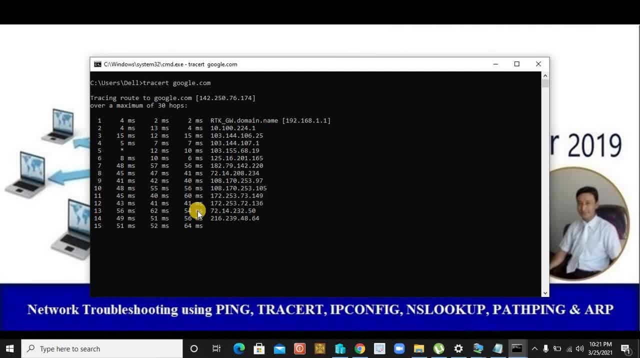 15. still it's counting now. that means we are passing through so many routers so that router itself means your hop count. actually 17 hops we have already counted now. that means tracer is over. that means, before i reach to this googlecom we pass through the 17 hops. that means 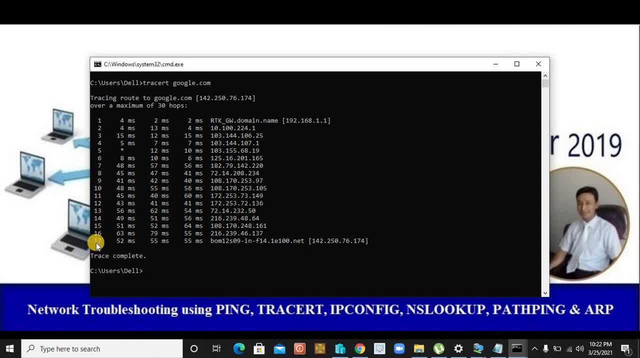 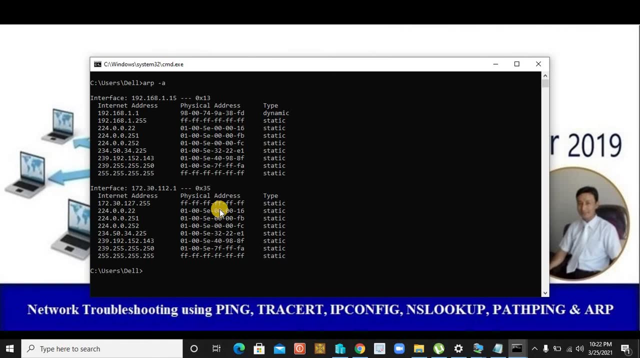 17 routers connection was successfully set. before we see or we meet the googlecom page. okay, now the next information that we are going to have. that means the next command line tool is the ARP. this ARP command tool is used to see the local address resolution protocol cache.